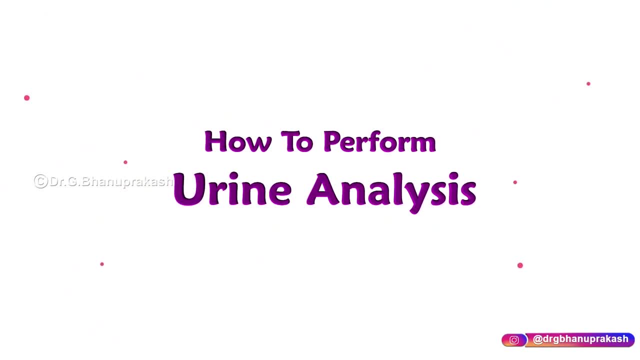 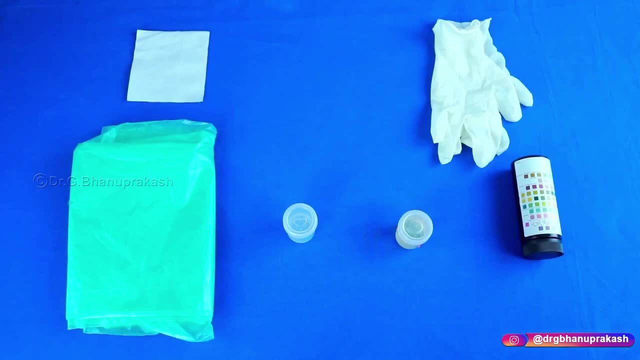 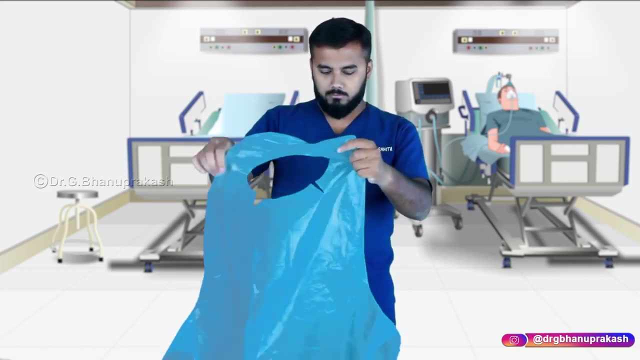 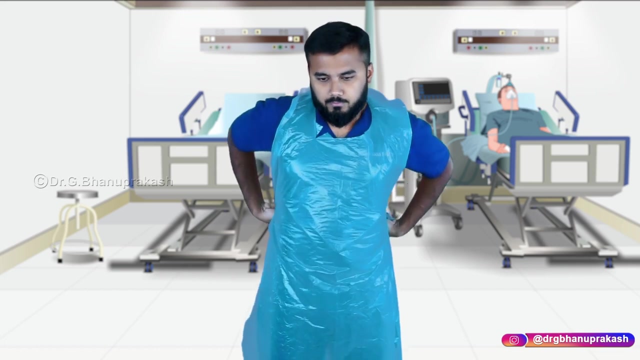 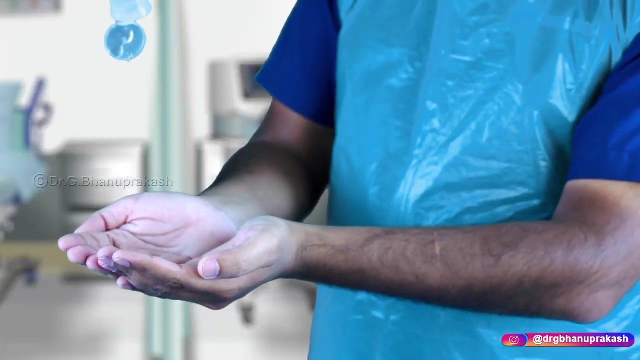 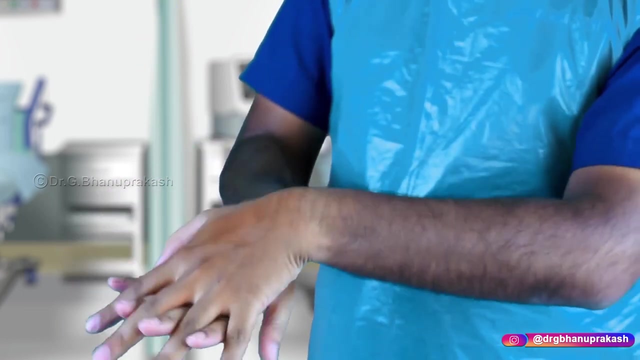 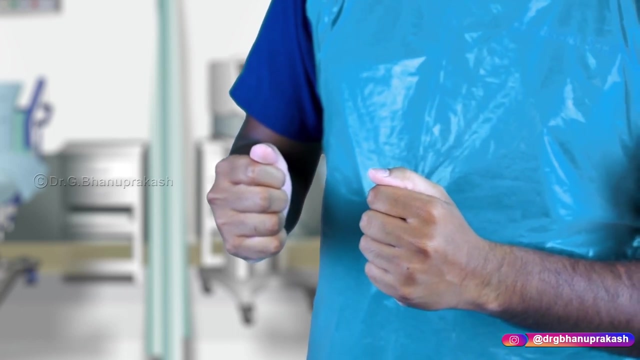 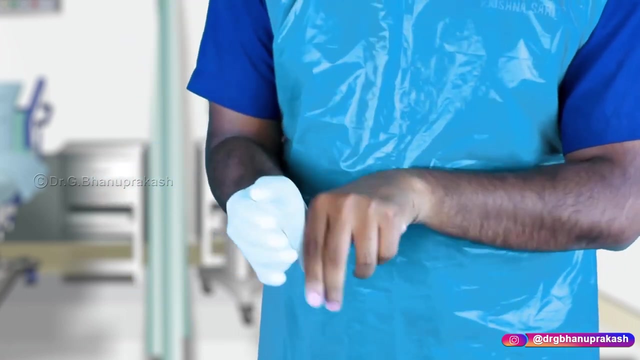 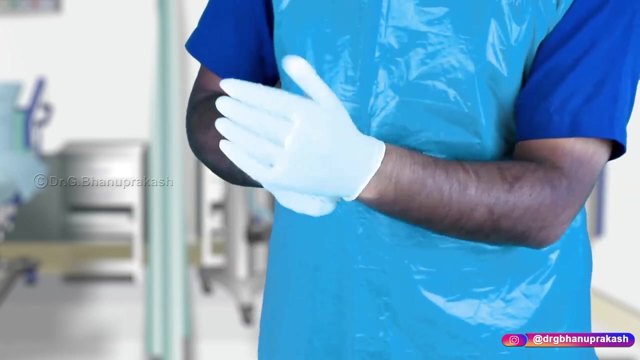 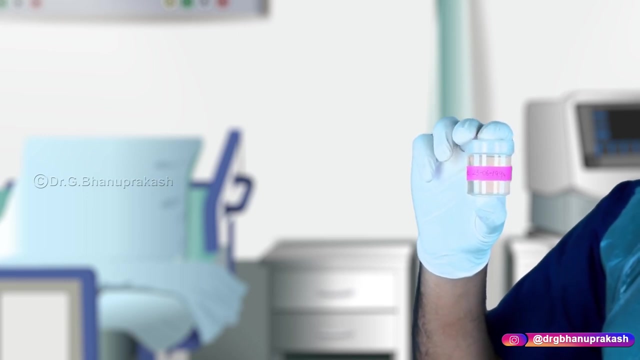 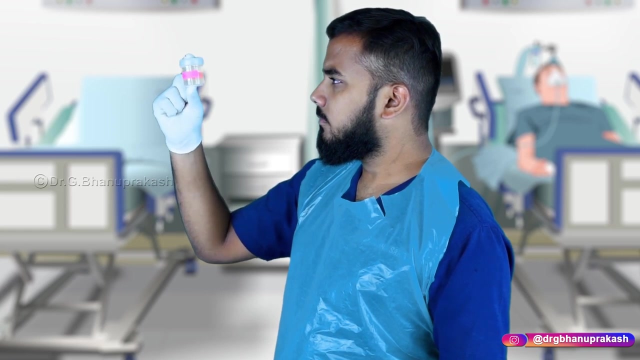 Thank you for watching you. after taking the urine sample, first of all confirm the patient's name. date of birth are most important, so check twice for the name as well as the date of birth. after taking the urine sample, carefully inspect the color of the urine, not only the color, even inspect. 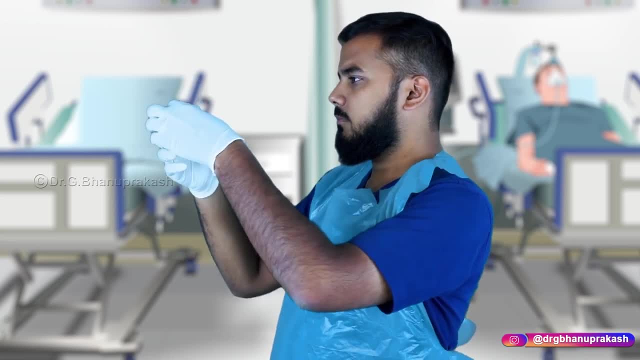 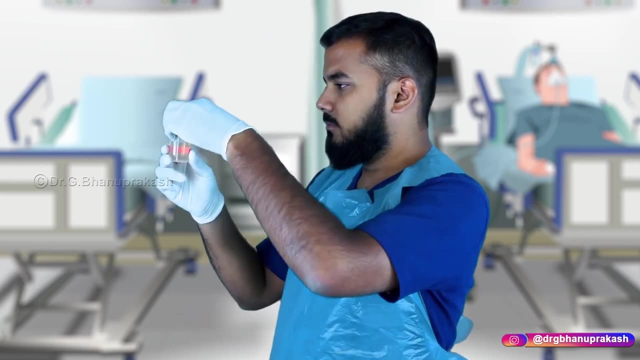 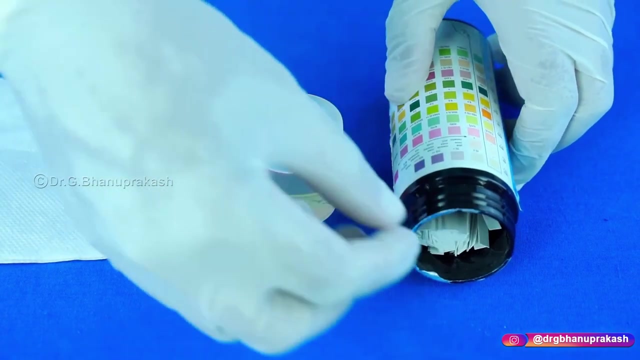 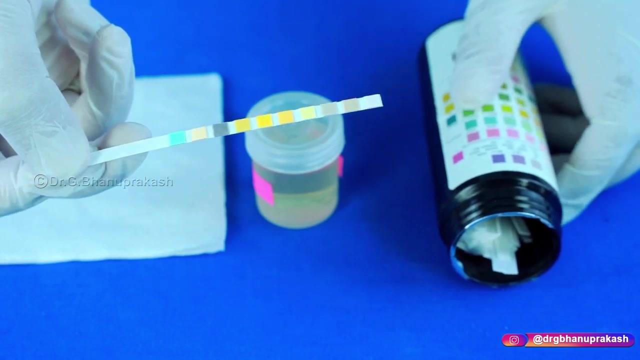 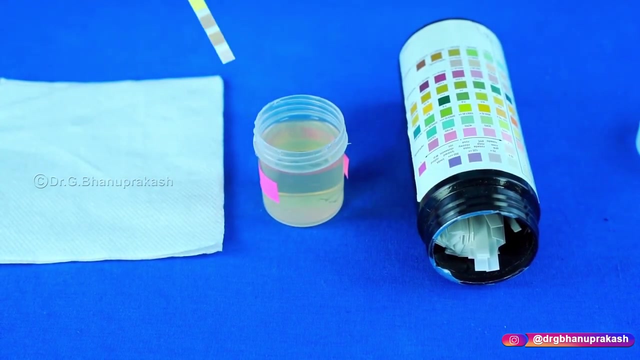 the clarity of the urine. after that, open the lid and now smell the urine. close the lid back and we are ready for the dipstick procedure. Take the dipstick from the box now. open the lid of the container that is containing the urine sample. Now immerse the dipstick into the urine sample container and make sure that all the zones 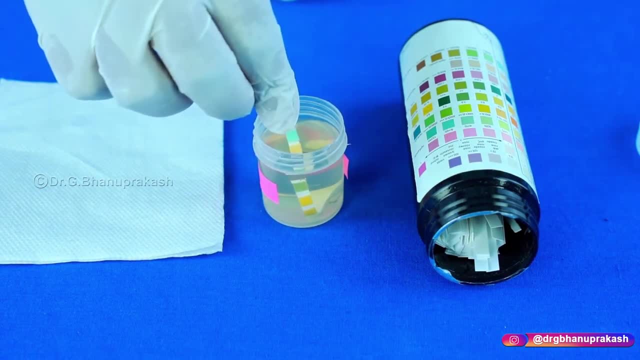 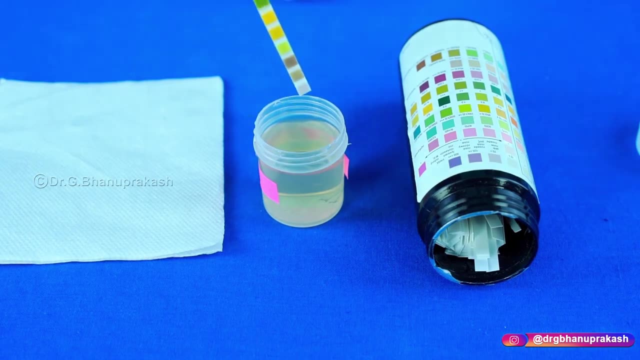 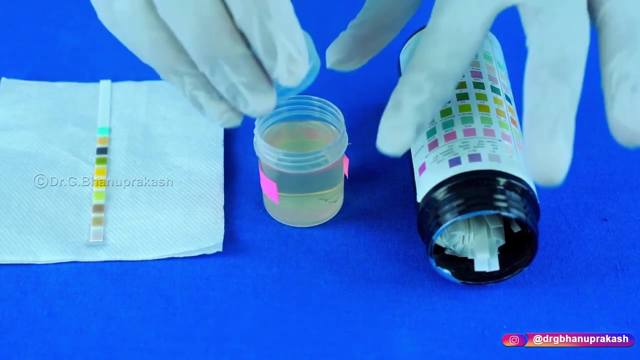 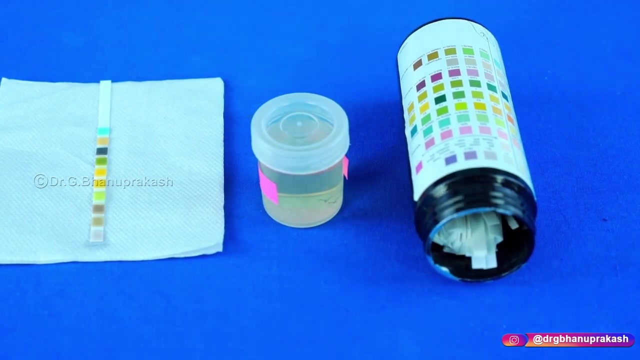 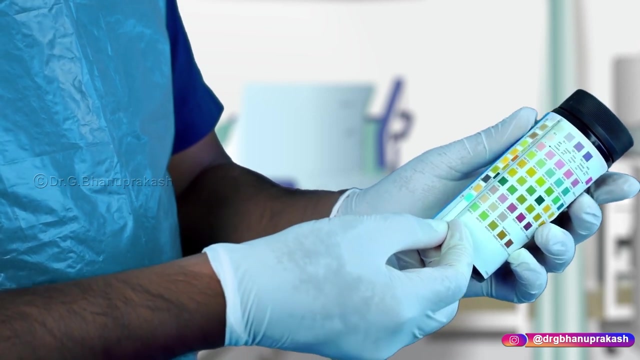 are completely immersed. Now remove the dipstick and place it gently on the paper towel. Now keep the lid back onto the container, wait for a minute and then start to interpret. Now interpret each test at the appropriate time interval using the dipstick analysis.